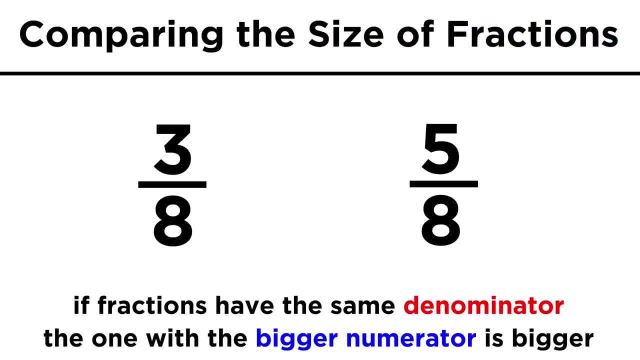 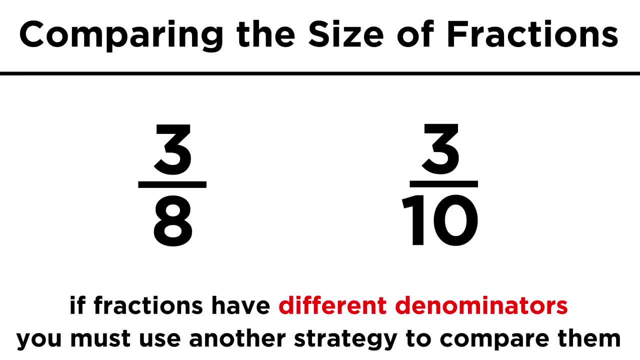 If two fractions have the same denominator, it is easy to see which one is greater. If the denominators are different, we can do a number of things. Let's say we are comparing three eighths and three tenths. Which is greater? 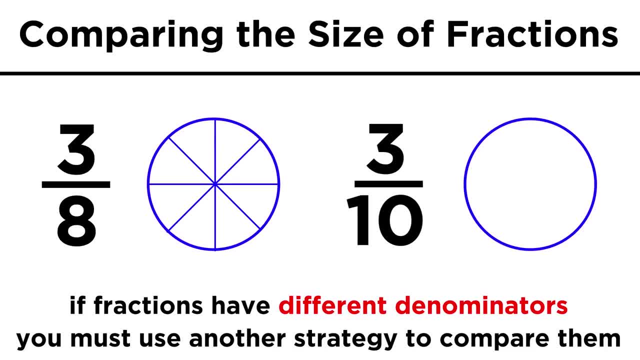 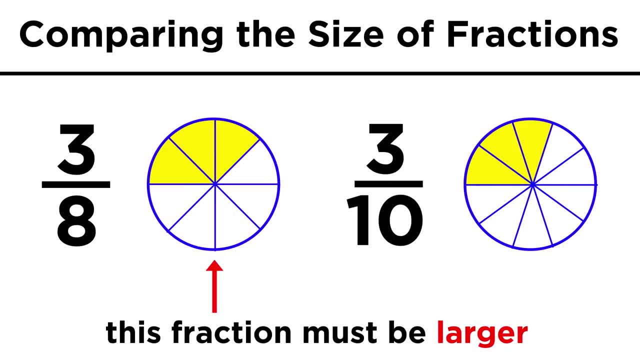 Well, let's draw two circles. One can be divided into eight pieces And the other into ten. Then let's shade three pieces in each circle. We can clearly see that three eighths covers a larger area, so it's the larger fraction. 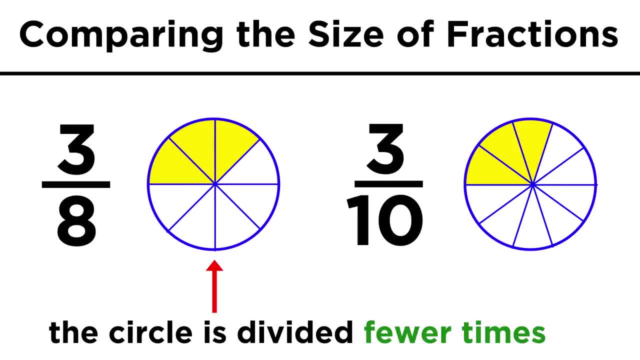 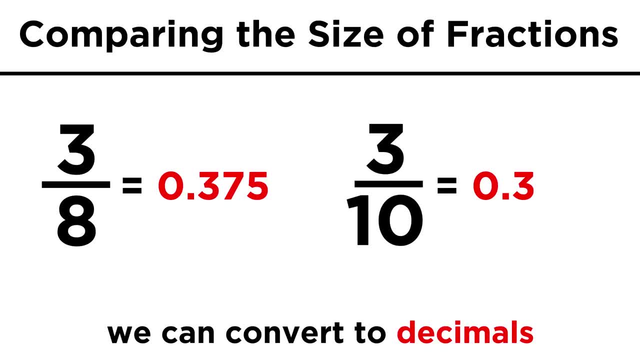 This makes sense because the numerator three is being divided fewer times than with three tenths. We could also do things like convert to decimal notation or find the least common denominator, both of which we will learn later. Of course, not all fractions are equal. 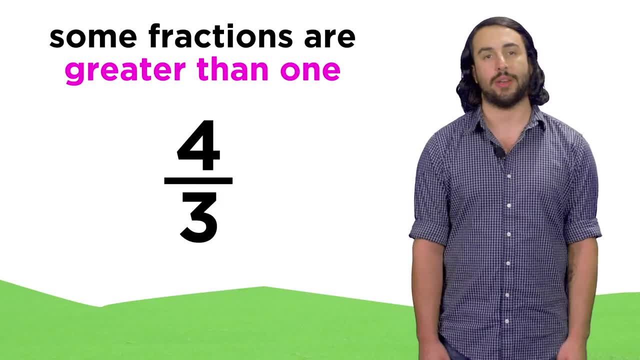 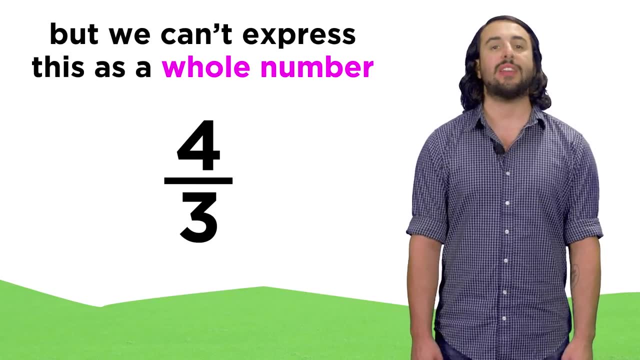 All fractions are less than one. Fractions can also be greater than one. This will be the case if the dividend is greater than the divisor, but the quotient is not a whole number. Take, for example, four divided by three or four thirds. 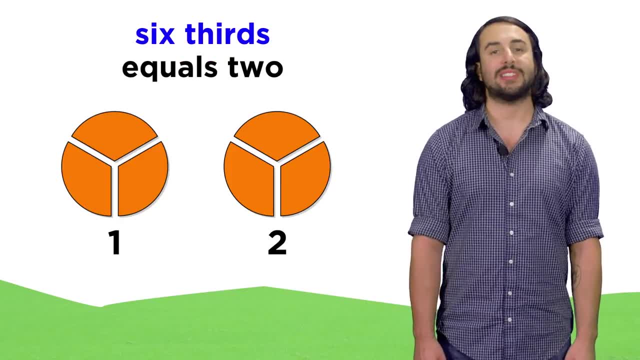 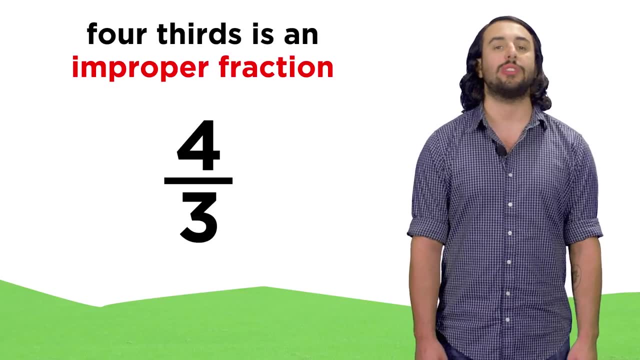 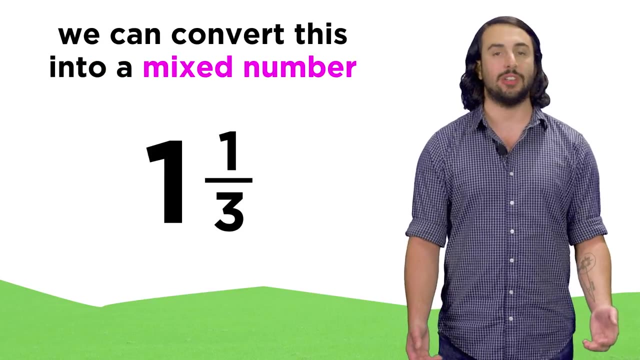 We know that three thirds would equal one and therefore six thirds would equal two. So four thirds is somewhere in between one and two. These are called improper fractions, and we can either leave these as they are or we, or convert them to mixed numbers like one and one third. 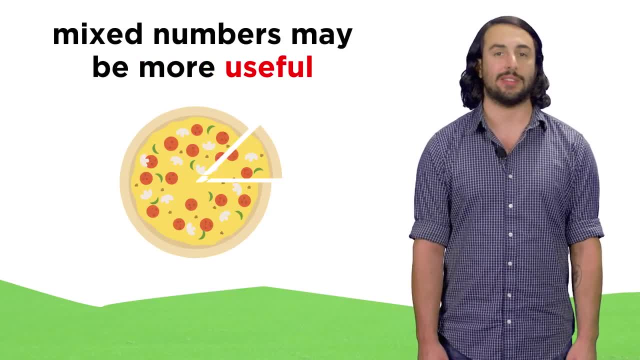 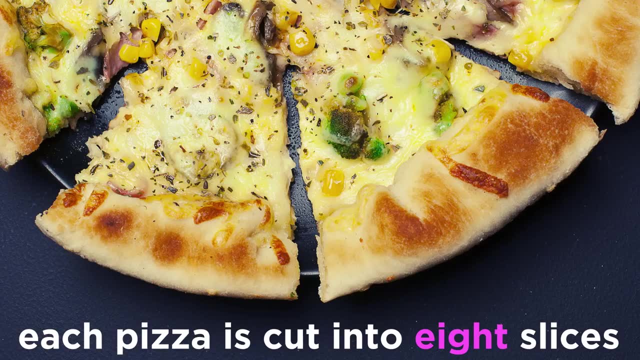 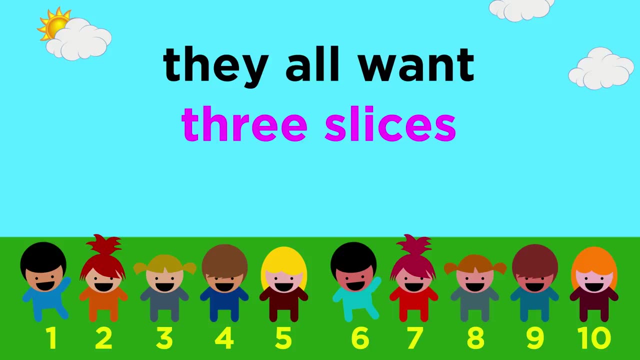 This can be useful in a certain context, like ordering pizzas. Let's say you're having a pizza party so you want to order some pizzas from your favorite restaurant. They cut their pizzas into eight slices and your ten friends each want three slices. 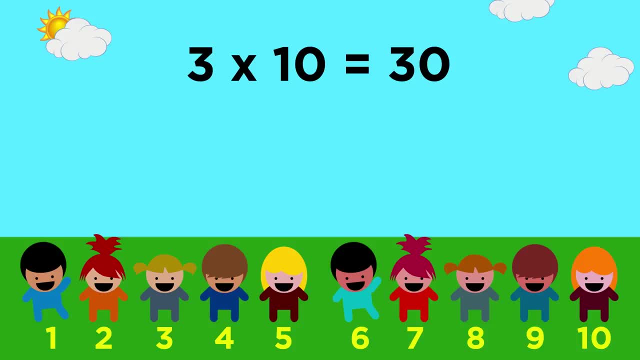 Doing the multiplication, three slices each times ten friends means thirty slices. Since each slice is one eighth of a pizza, we could say that we need thirty eighths of a pizza, But when we call to order we wouldn't say it that way. 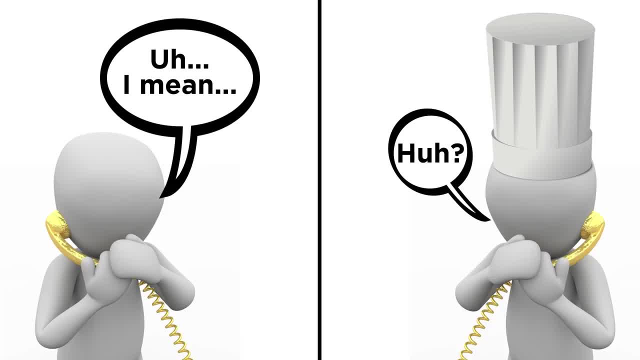 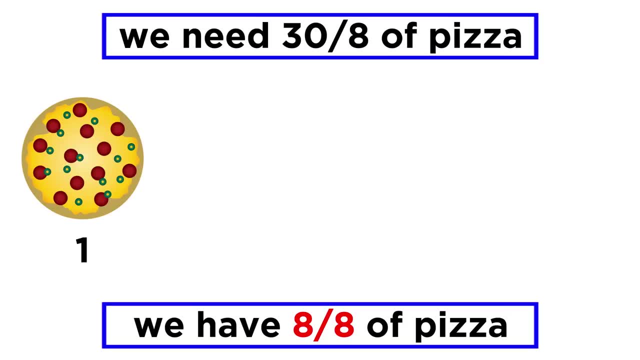 We need to order a specific number of whole pizzas. So how many do we need? Well, eight eighths comprise a whole. so eight eighths is one pizza, sixteen is two pizzas and twenty-four is a pizza. So that gives us three whole pizzas.